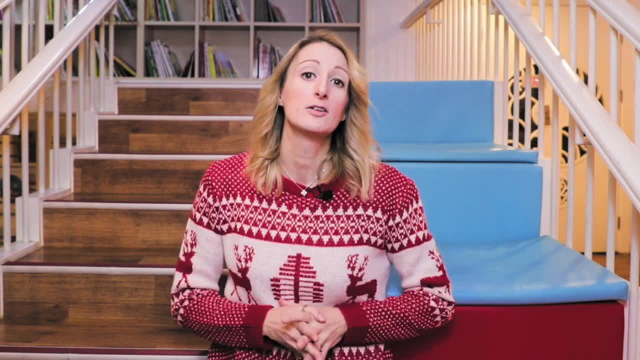 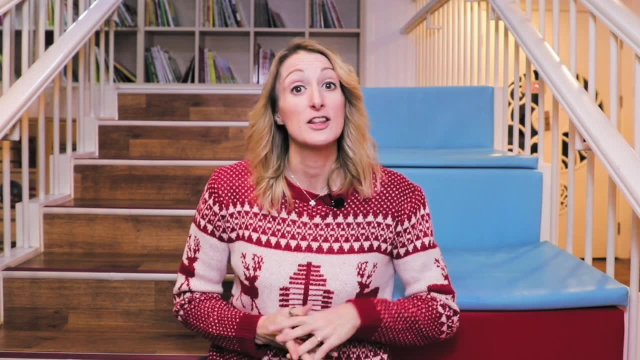 and the how, The what is what we should be teaching and what we can realistically expect from our students. I mean, you wouldn't expect a three year old to count to 100,, right? The second is the how, and actually there are three steps to teaching numbers. So let's take a look at the first step. 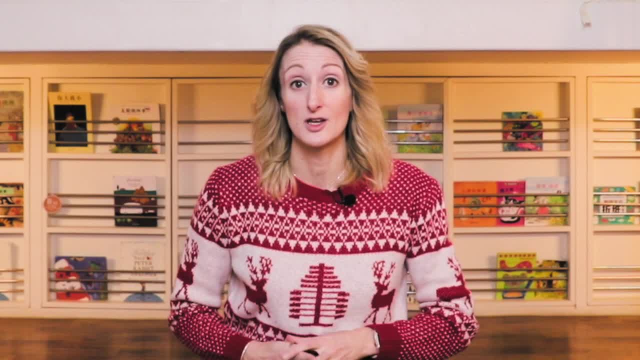 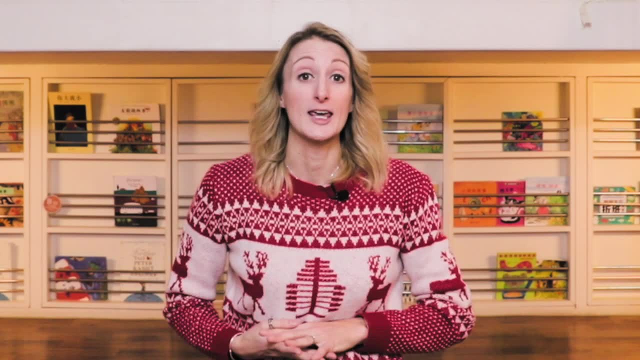 sequence. What I mean by sequence is the order in which numbers go. so we know that counting goes 1-2-3 and not 2-1-3.. For us this might seem obvious, but for students learning to count for the first time it's. 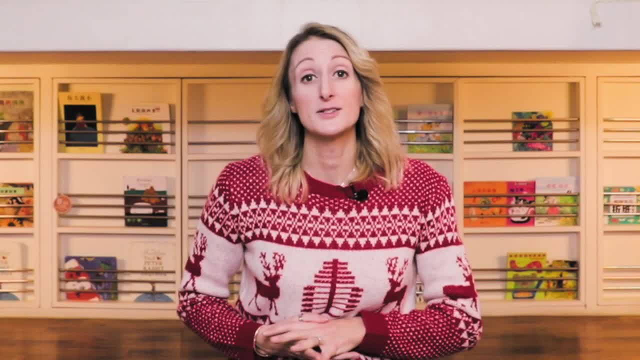 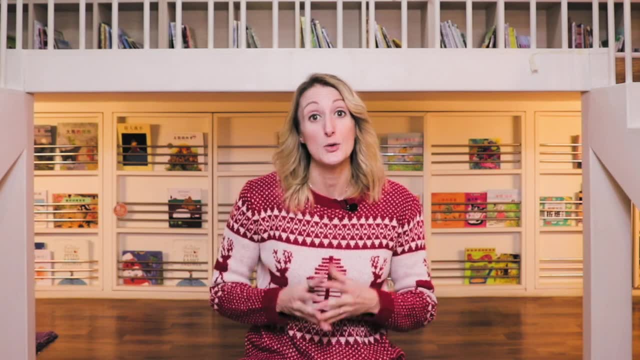 not, and they need to learn it. So how do we teach this? Well, practice makes perfect, and we can practice counting all the time. Like a lot. Take a moment to stop and think about all the different opportunities you have during class to practice counting, Maybe. 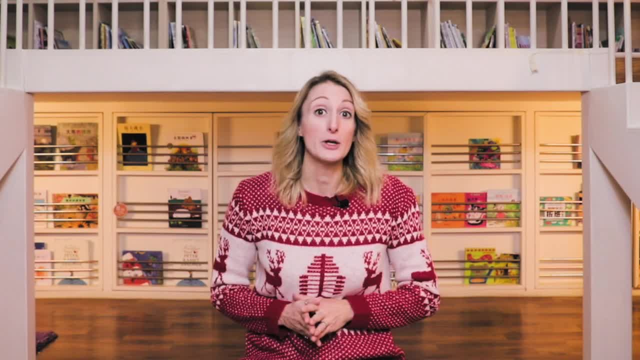 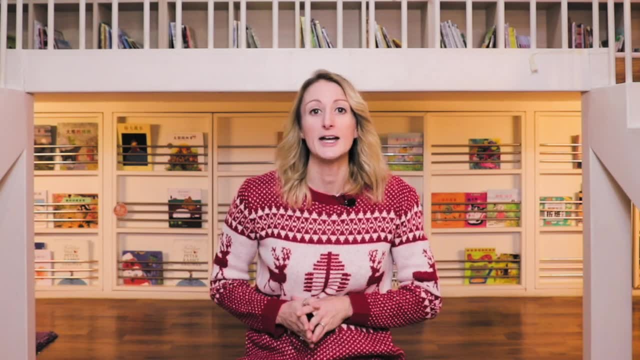 you're laying out some flashcards and you can count as you go. If you're teaching body parts, you can count your fingers and your toes. If you're teaching shapes, you can count how many circles and how many squares there are, Even just lining up and waiting. 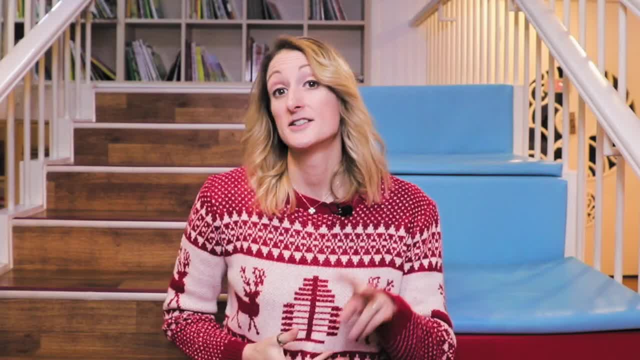 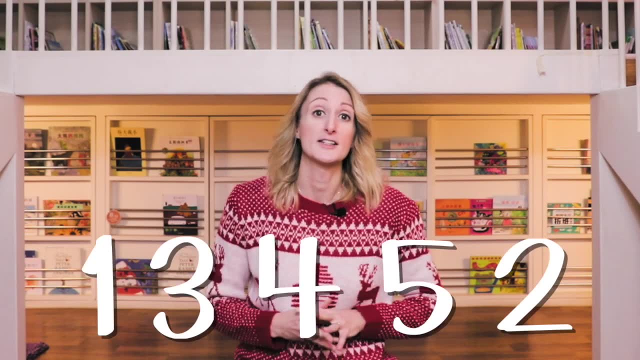 to go outside. you'll be surprised how much fun students find counting. Step number two: number recognition. Now that students can say their numbers, they need to better recognize them on paper. A great exercise for this is to have students put number flashcards in the correct order. I've given a great example of this in part two. 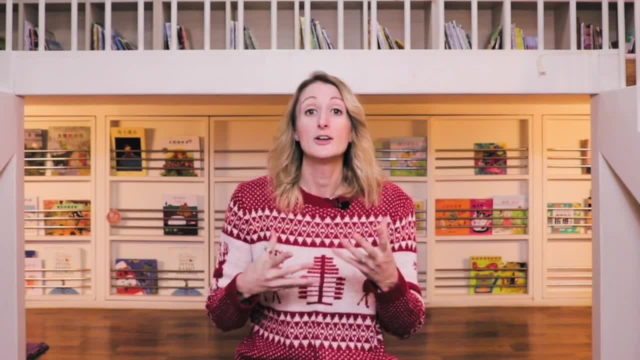 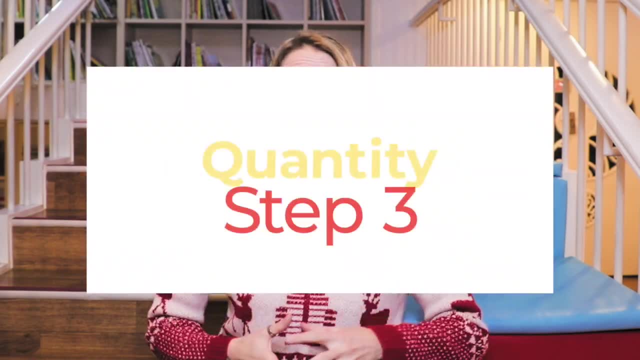 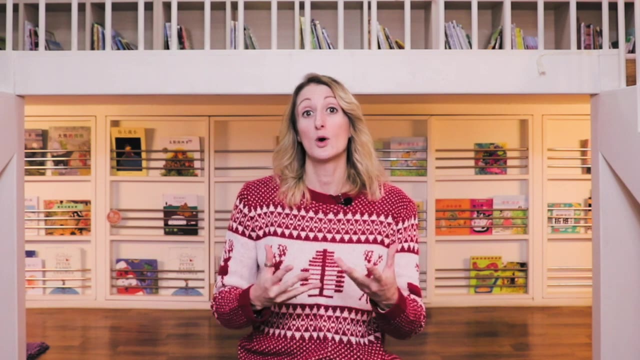 of this number series. Just like learning any other word, learning to recognize numbers takes time and effort. Step number three: quantity. The final part of the puzzle is quantity and matching numbers with it. What I mean by this is that students need to understand the quantity that numbers. 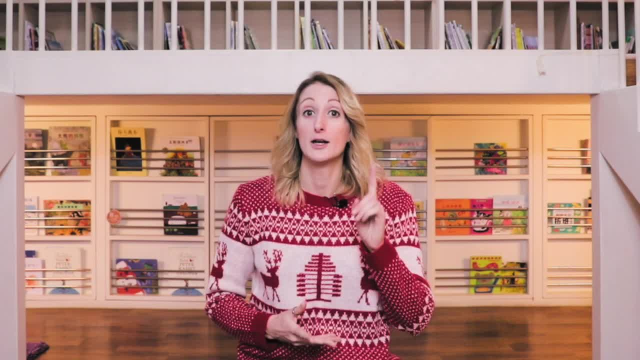 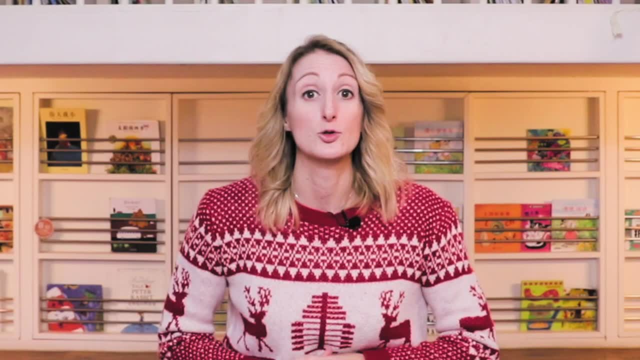 represent. So if we were talking about candies, for example, then number one would represent one candy, number two would represent two candies, and so on. If students have really grasped quantity, then they should be able to correctly count the number of candies in. 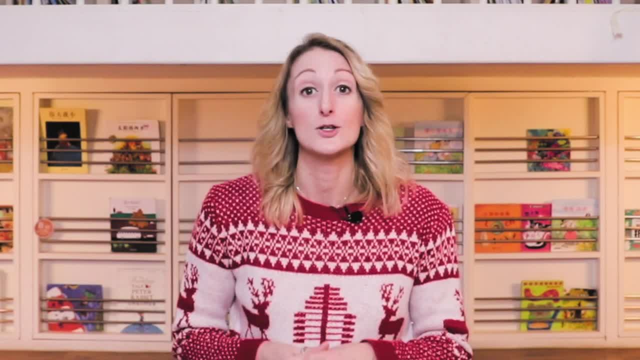 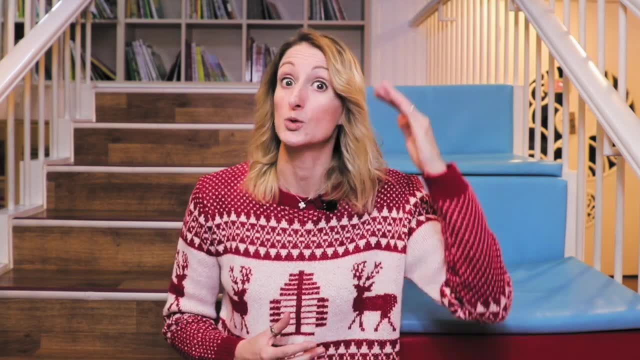 a jar and correctly count out a given number of candies. So now that we know the three steps to teaching numbers, we need to understand what we should be teaching students so that we don't teach way above their level. So let's take a look. 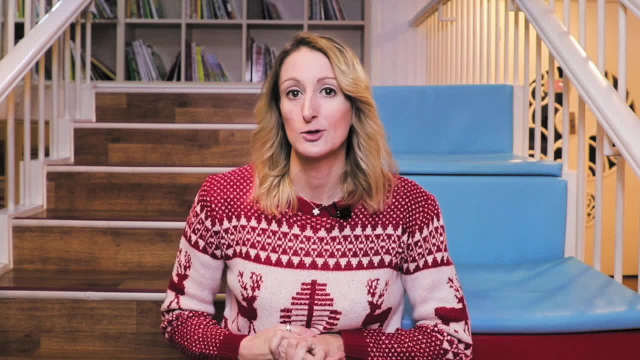 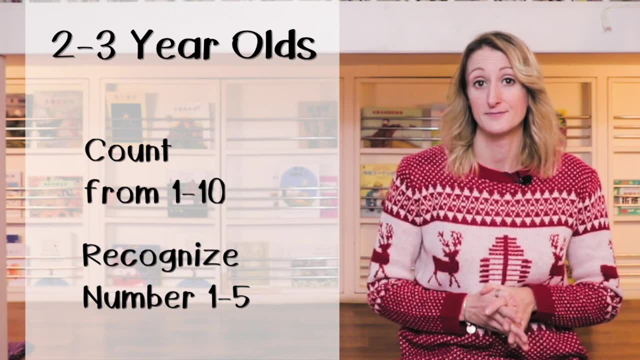 at some different age groups and what you can expect, Starting with those two to three year olds. Oh, the little darlings. These little darlings can count from one to ten and recognize numbers from one to five. Three to four year olds. little munchkins, These little munchkins. 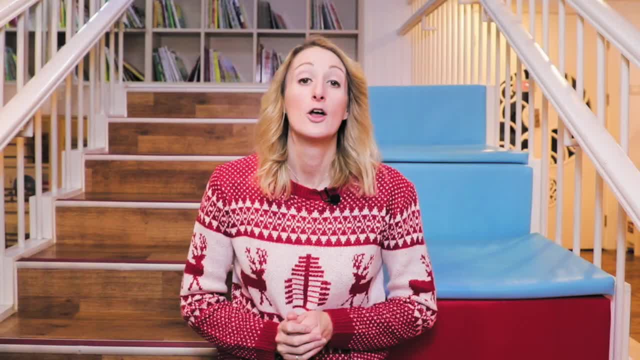 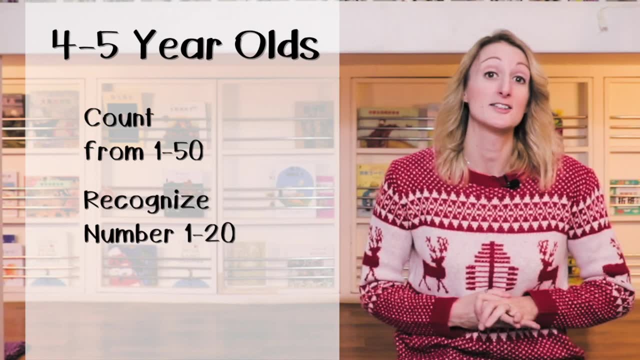 can count all the way to twenty and recognize numbers from one to ten, Four to five year. the bigger little ones, These little darlings, can count all the way up to 50 and recognize numbers between 1 and 20. but not only that: at this age they can. 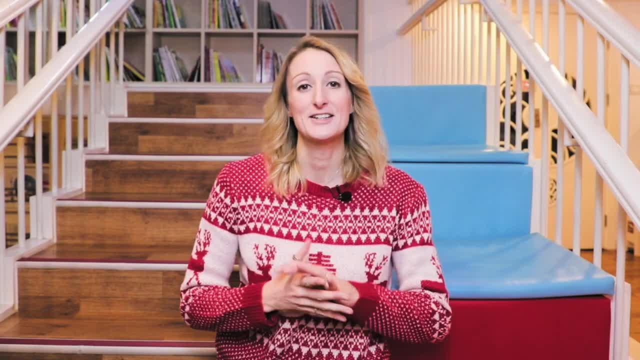 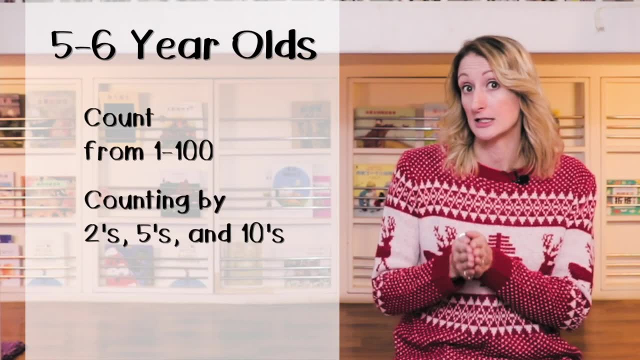 also start counting backwards, from 10 down to 0.. 5 to 6 year olds, the big little ones, These little darlings, can count all the way up to 100 and can even start counting in twos, fives and tens. At this point they can also start adding. 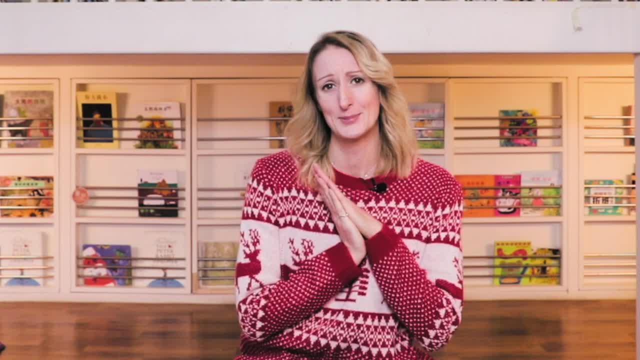 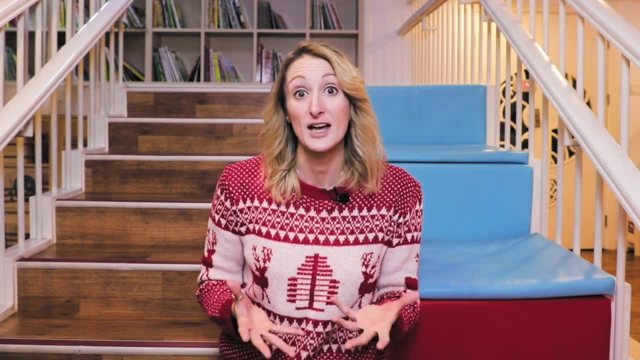 and completing some simple math. Oh, it's like they've all grown up. Of course, this is all just a guide, and you are going to encounter some students who have been exposed to numbers much earlier and therefore develop their mathematical reasoning skills much faster. On the other hand, you're going to encounter 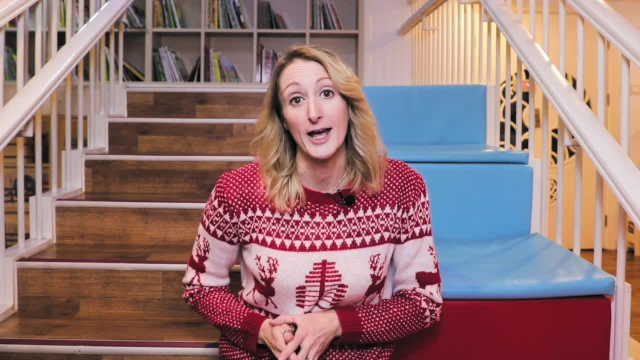 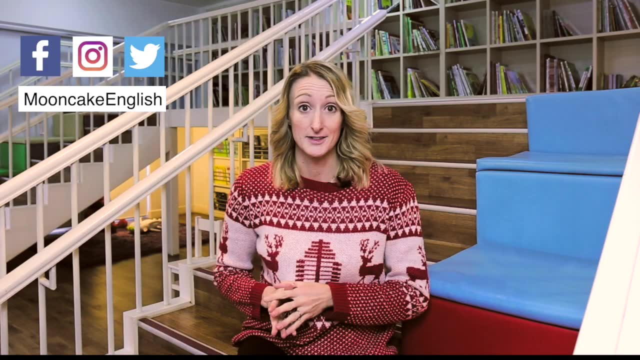 some students who are learning much slower. That's all okay. just make sure that you adjust the level for the class that you're teaching. So there you have it, everything you need to know about planning your numbers class. Be sure to check out part two, where I go through some more practical ways of how to teach. 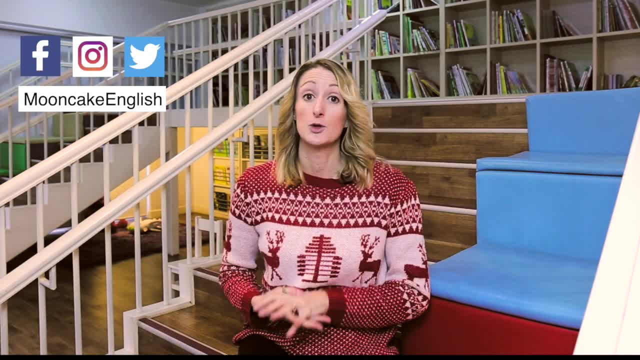 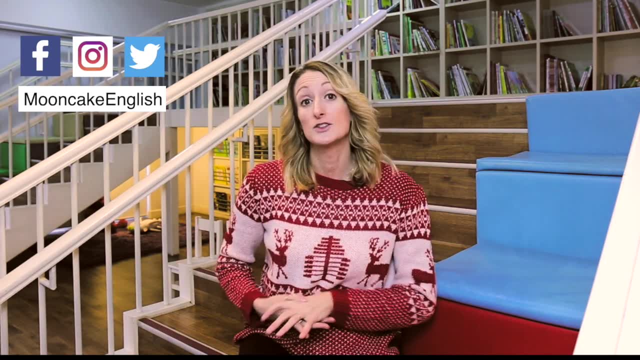 this in the classroom. If you like this video, let me know by commenting with the word helpful in the comments below And by sharing with your fellow teachers. If you're looking for some more fun ESL games, then you can check out some of my other videos right here. That's it for 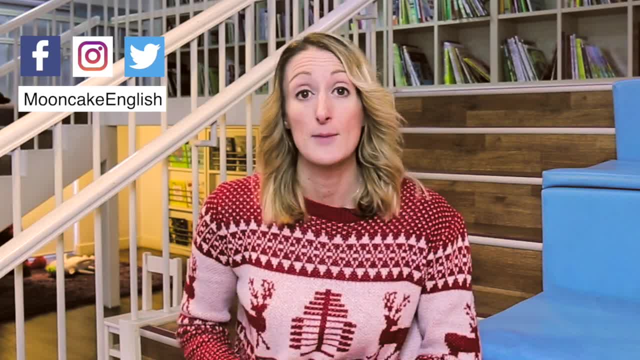 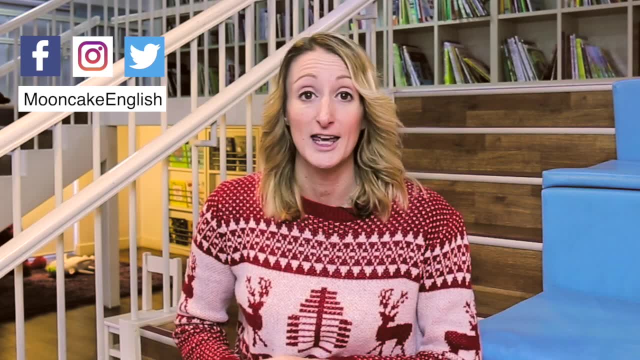 this video. thanks so much for watching. You can find me on Facebook, Instagram and Twitter, or, if you're interested in a Mooncake sweatshirt or mug, you can find them linked below. And, of course, remember to subscribe and hit that notification bell for more weekly ESL teaching tips from Mooncake. 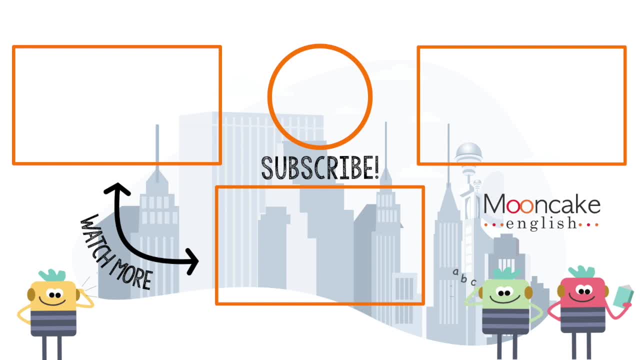 I'll see you in the next video. bye, bye.